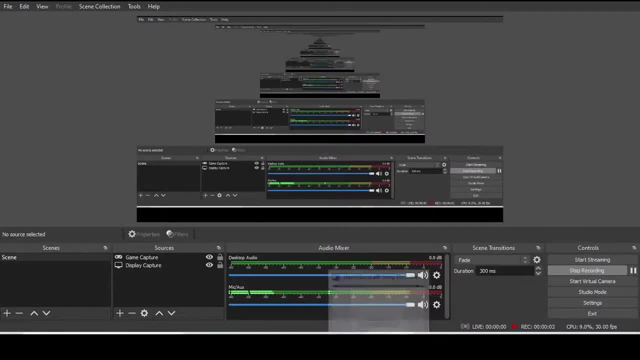 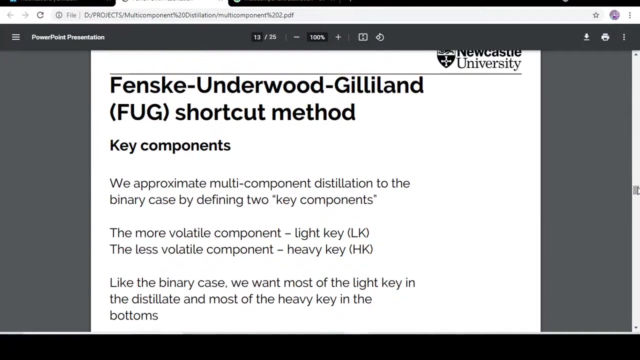 Hello everyone, In this video we will be learning the designing of multi-component distillation column. Basically, we will be learning the shortcut method for designing the multi-component distillation column, which is FUD method. So if anyone of you knows about FUD method, FUD shortcut method is that we categorize two of the components, of all the components in the mixture, as a light key and a heavy key. 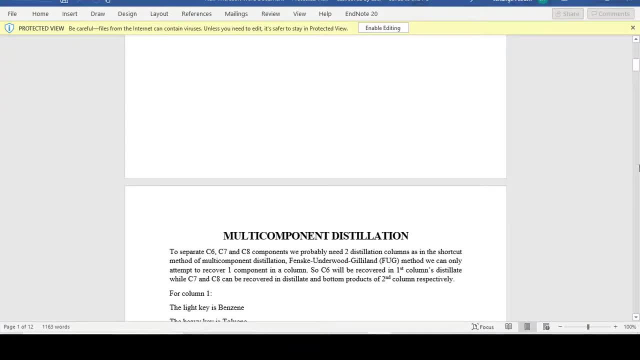 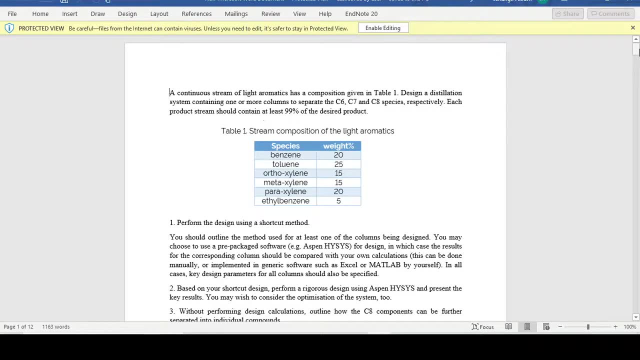 Consider an example in which we have following component mixture And we want to separate it. We want to separate benzene out of the mixture, as this is clearly not a binary mixture. So what the shortcut approach does is that it separates one of the components from all the components in one column. 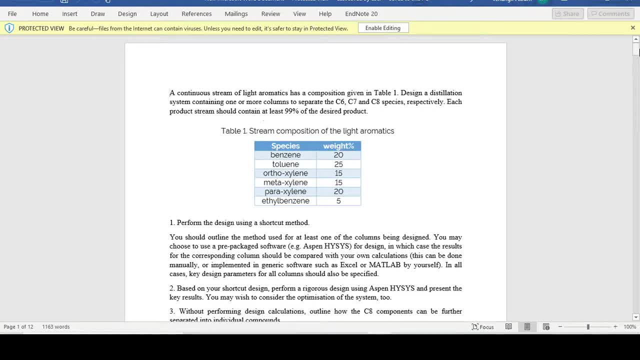 Like it won't be possible. it won't be designing a multi-component distillation column which will be simultaneously separating all the components, But it will be separating only one component with various components, So it will be separating all the components. So it will be separating all the components. 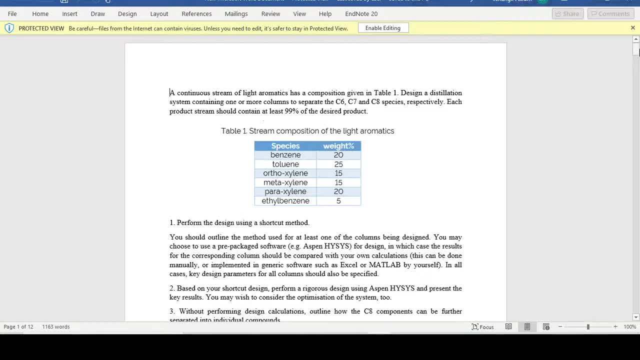 So it will be separating all the components And we want very high concentration, either from the top or the bottom. So what this approach does is that let's say we have the following mixture And we want to separate it. First of all, we have to know basically…. 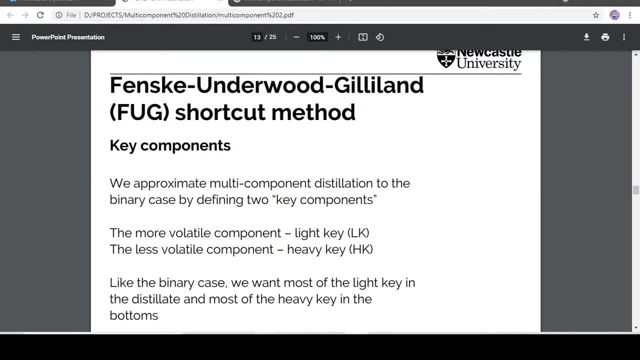 Just a minute. let me combine… I have this one and this one… If I go straight together and I fill, Since we have more than 100 components in this mixture, then this one is very curse. When we mix the two components together, one of them will become one. This is how it's going to turn out. So this is the functions of the mixture. Now another process: how to make itons in this 말씀드�ing in this further in next part of the video. 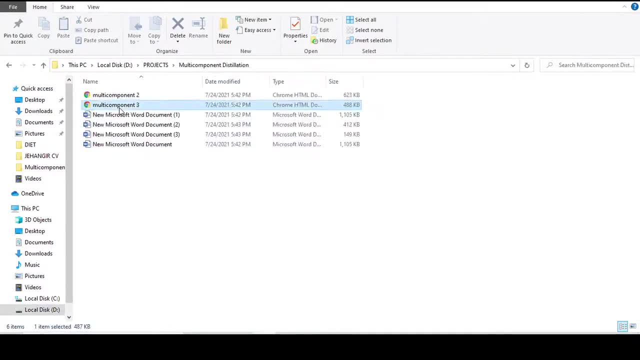 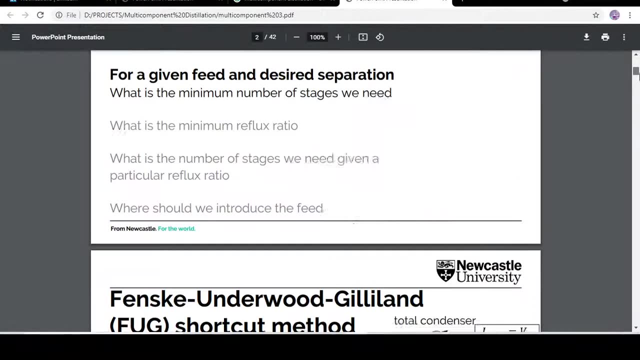 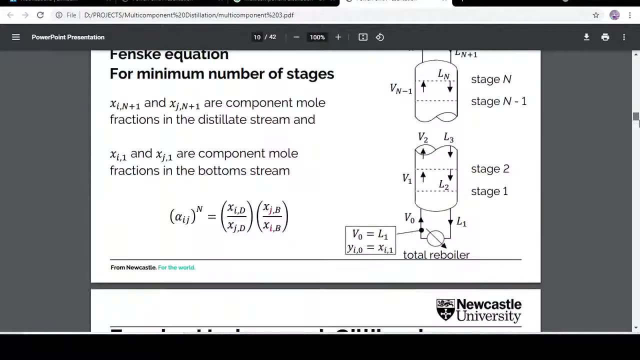 One other thing is that when we mix quality ingredients together, then this new method might become more00 effort a minute. let me so basically a few. G method is used to design a multi component distillation column and it is basically a combination of three equations: F, F. 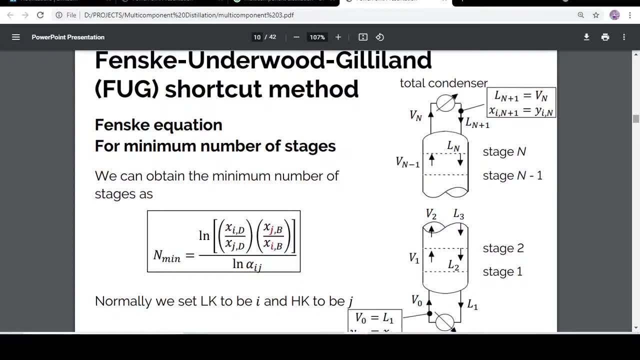 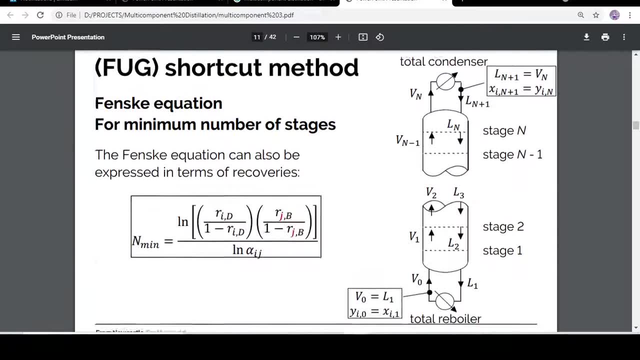 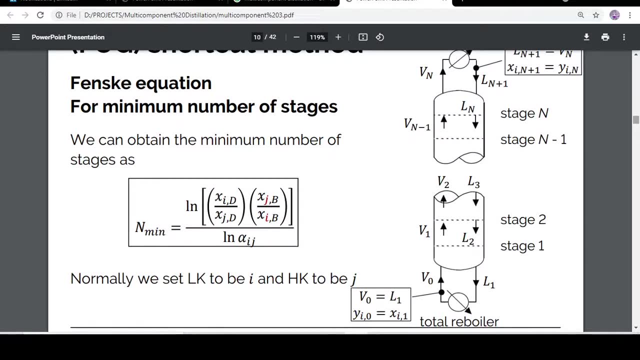 means Fenske and Fenske equation determine the number of minimum stages required for a multi component distillation. similarly, and you can, I can elaborate the equation as well, like it's the ratio of log of two parameters: in denominator we have the quality volatility, while in 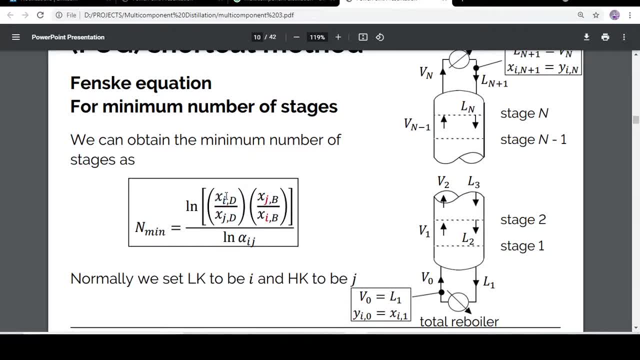 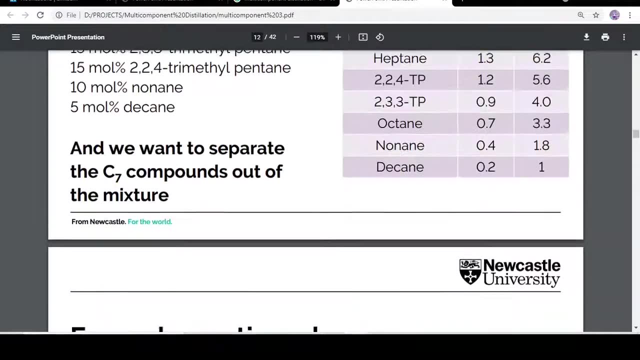 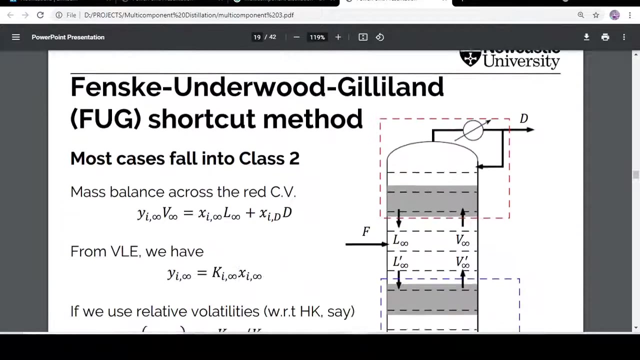 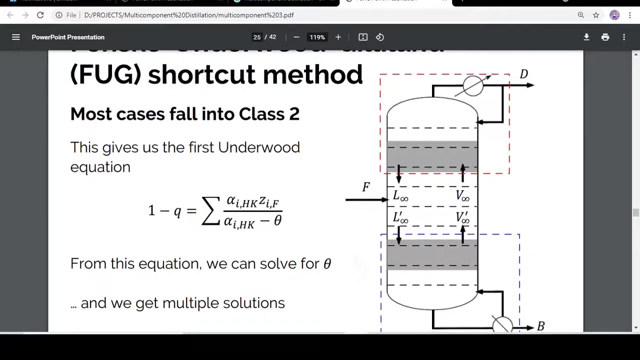 well, above we have the mole fraction of two components, which is I and G. I basically light key, and J is basically the heavy key. I will explain these parameters later, but let me first briefly explain what these equations are. so we have seen the Fenske equation, now let me open the Underwood equation. okay, 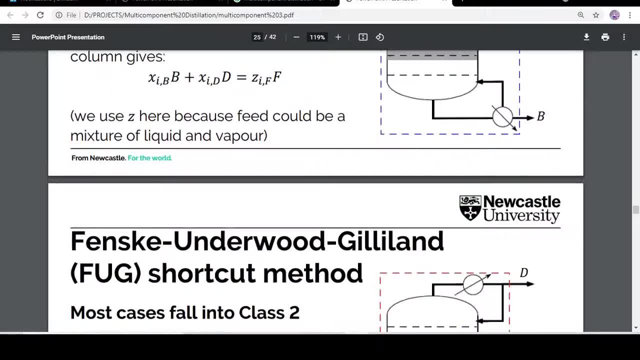 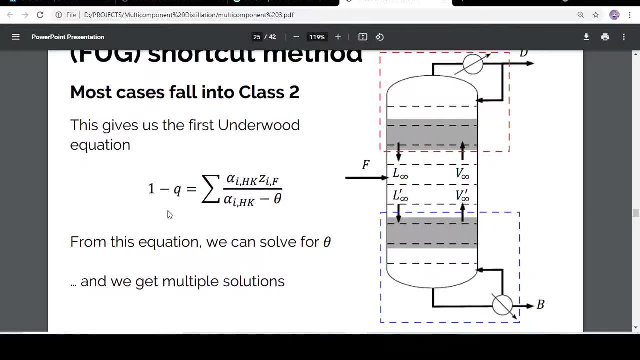 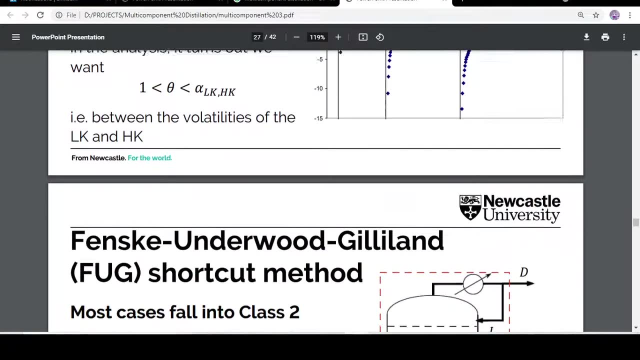 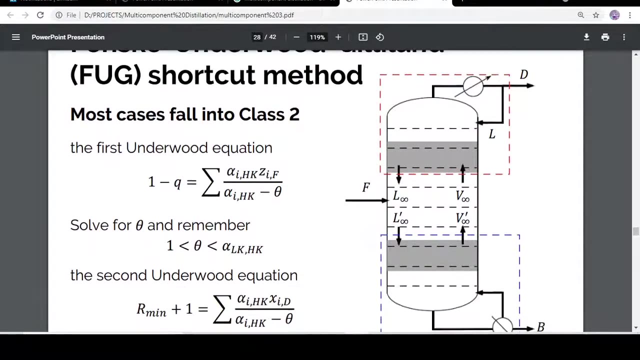 this is the Underwood equation. so basically, Underwood equation is a combination of two equations. this is the first one, as you can see that we will solve for theta in this equation and based upon the assumptions okay. and this one is our second equation, after solving for. 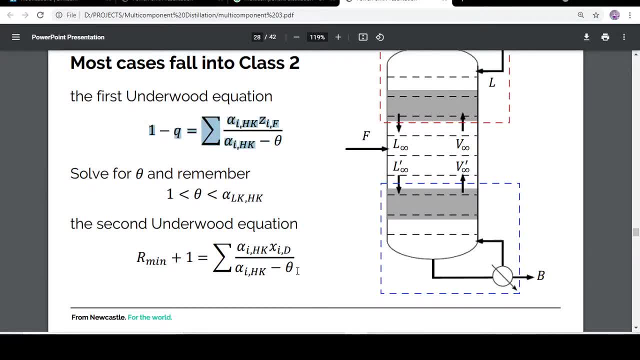 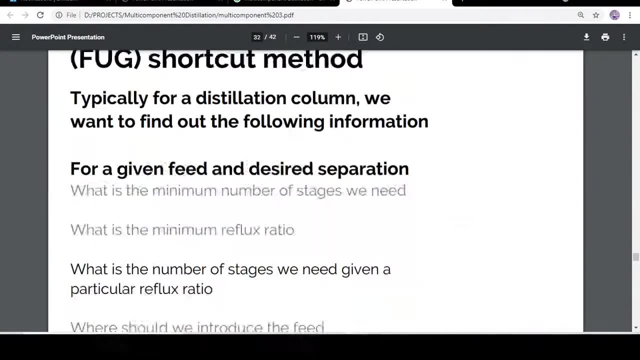 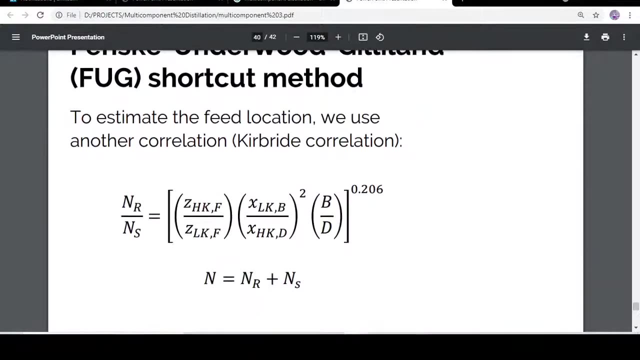 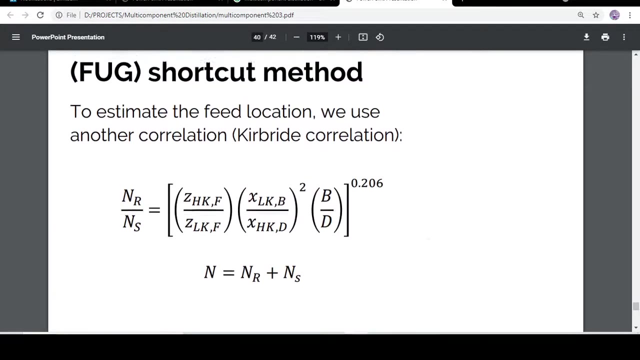 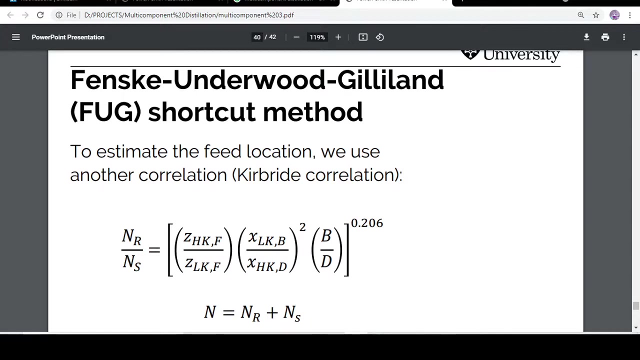 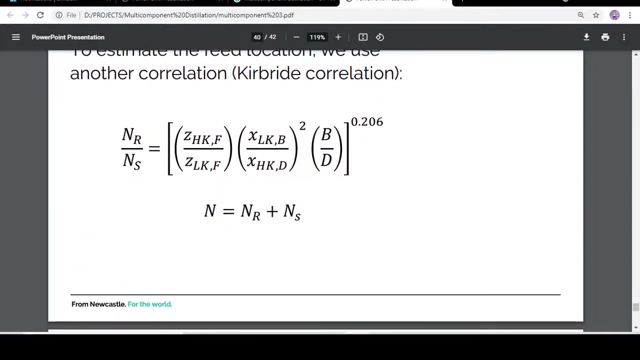 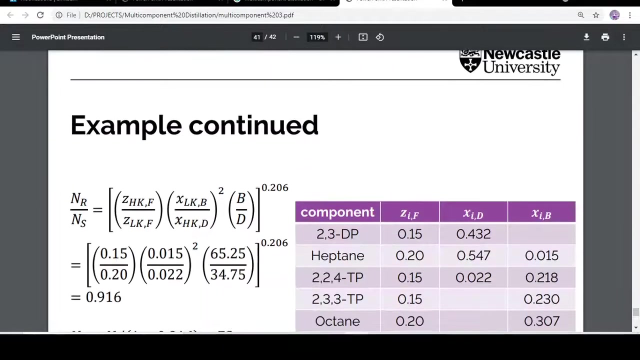 theta, as all of the parameters are known by us. we will be calculating the minimum reflection for our bigger number of degree equation. normal veio, let's say雨- I don't know how to pronounce it, kid bride, correlation and it's you. and it's used for the determination of feed feed stage. basically, like we calculate the 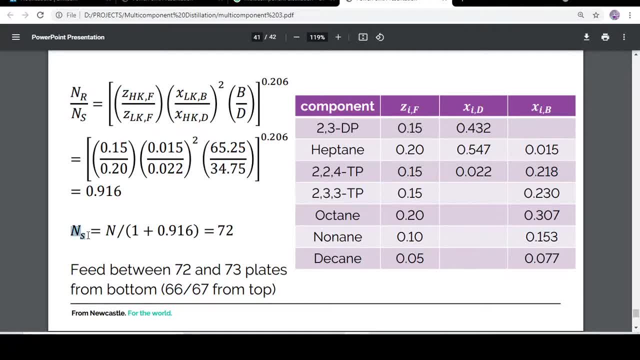 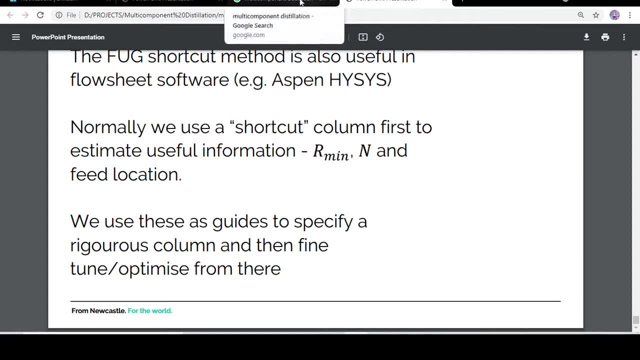 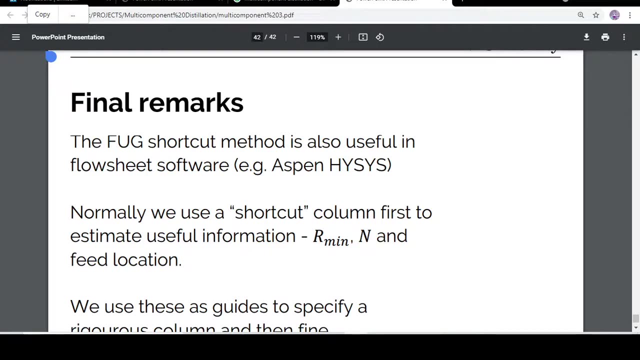 ratio and after calculating the ratio we can find the feed stage which is given. okay, this method is also used as a computer from Manchurian, such as in Aspen high city. it's basically used in the shortcut distillation pellet of distillation, of distillation in Aspen, high seas. those who have viewed aspen. 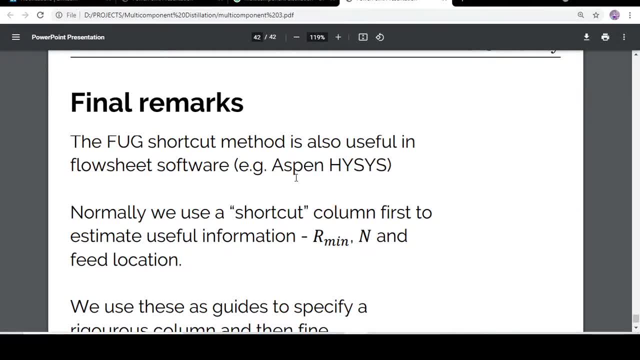 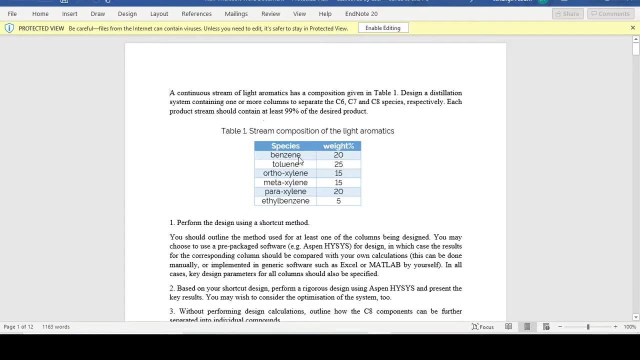 high seas, know about it and I will also show you how to use it in Aspen high sea. that what we get if we solve manual way and what will we get when we solve it in Aspen high seas. so let's say we have a component mixture of benzene, toluene and xylene, so basically xylene. 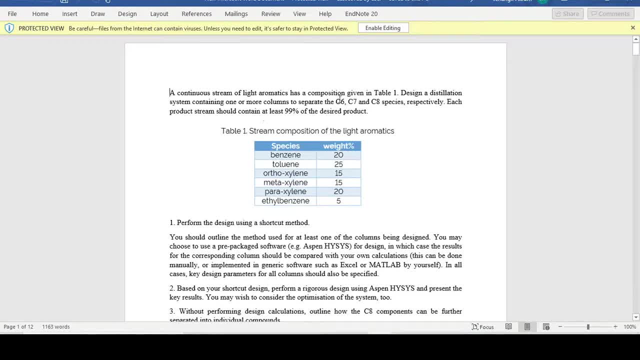 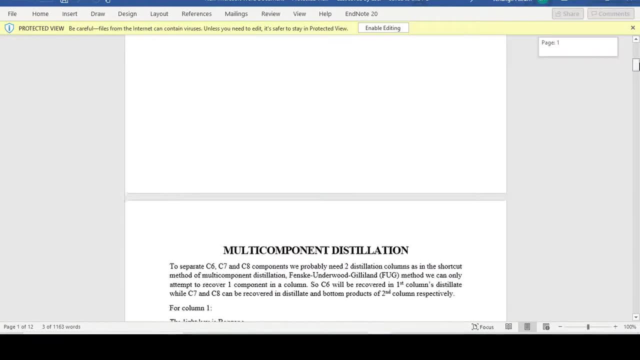 and ethyl benzene or c8 component. so we are required to separate c6, 6, 7 and c8 components. it will require us to distillation column to separate them. so we have. we know that we just have to use those three equations. it's not. 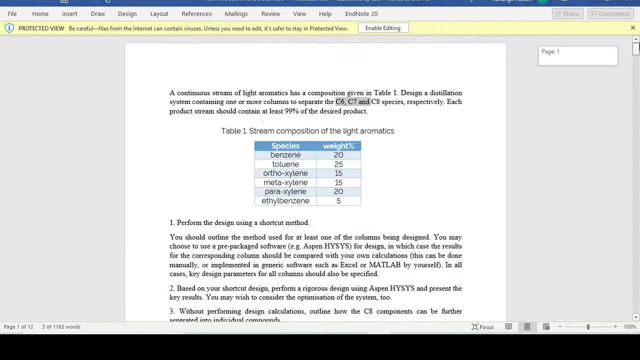 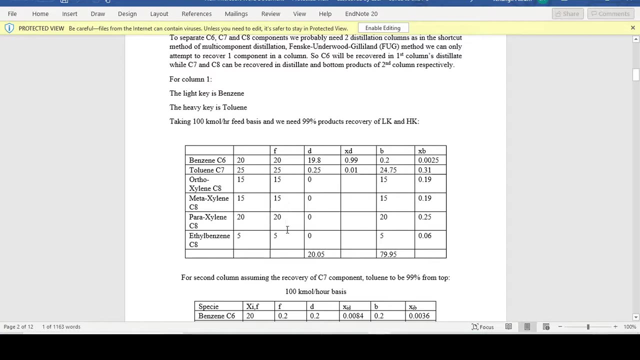 different, that rocket science behind understanding. and we had understanding them. I will elaborate them briefly. let's say we want to get 99% separation of each component. first of all, we will draw a table in which we will specify the composition of the feed. we will select a key component- let's say we select light component to 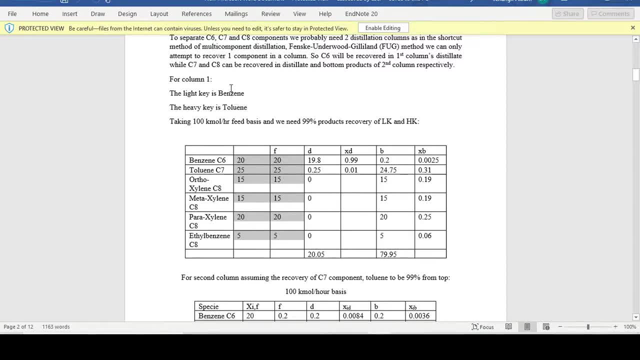 be balzean and heavy component to be tal потер main. you should know that light component is not necessarily the lightest component. it can be any component which we, you, which we- to choose to carry out separation, based upon which, aí which is named as heavy component, it is. it is also not. 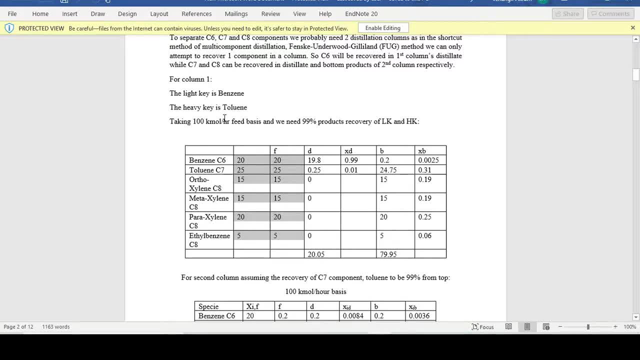 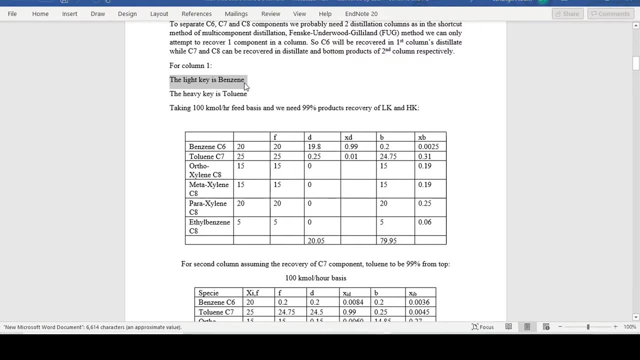 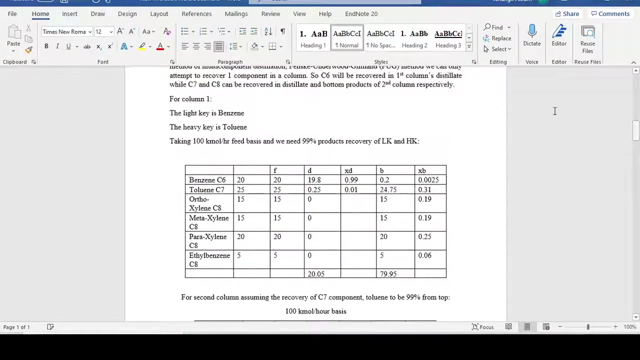 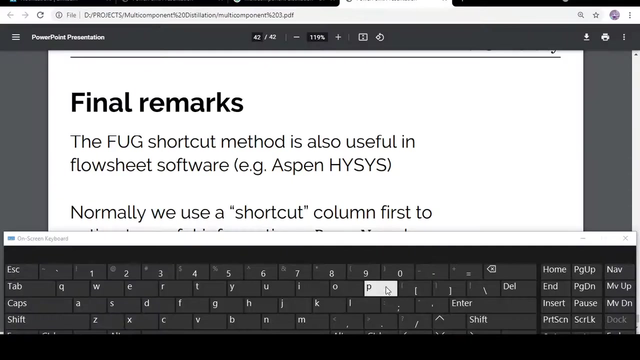 of course, heavier than the light key. all other components are termed as non-key components. so after selecting two components, we will be carrying out our calculations. also know that we can say that we can write that light component is basically- will be basically i in our calculations and heavy component is basically. 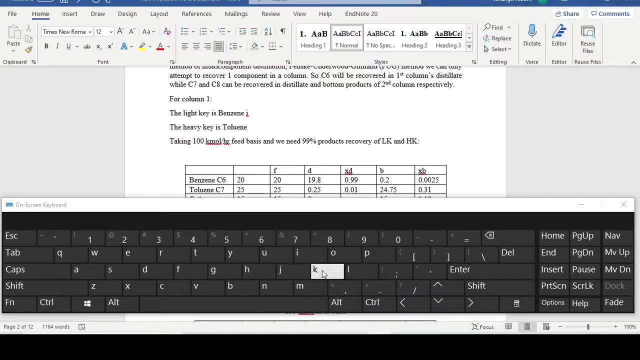 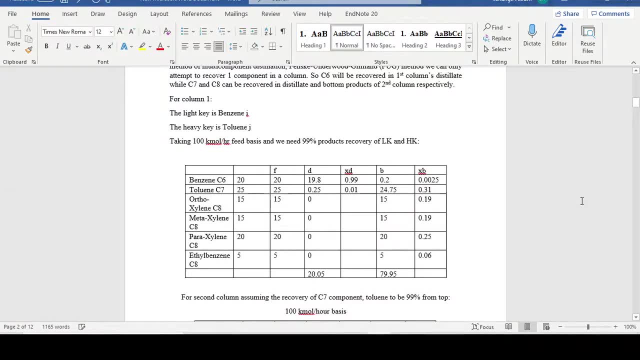 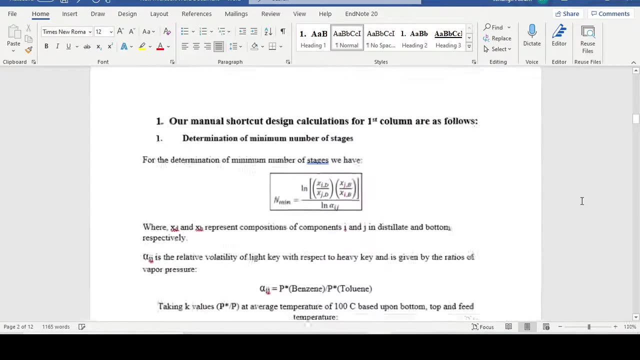 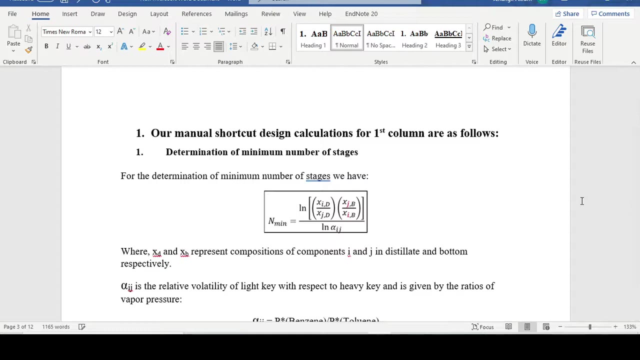 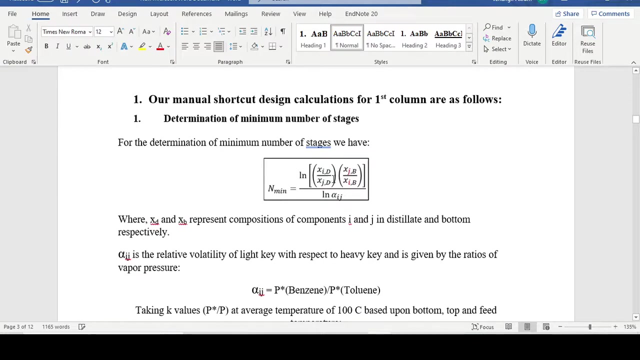 j in our calculations. okay, i am defining so it won't be difficult for you once you will go through the file. okay, what we do is, first of all, we determine the minimum number of stages that are required to separate our component mixture. okay, so what we have in this equation is: minimum number of stages is equal to ratio of logs, as i have. 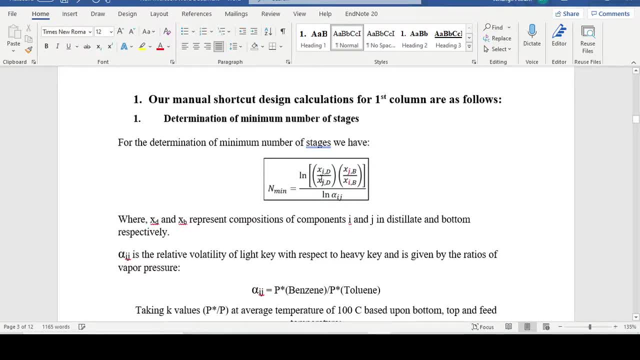 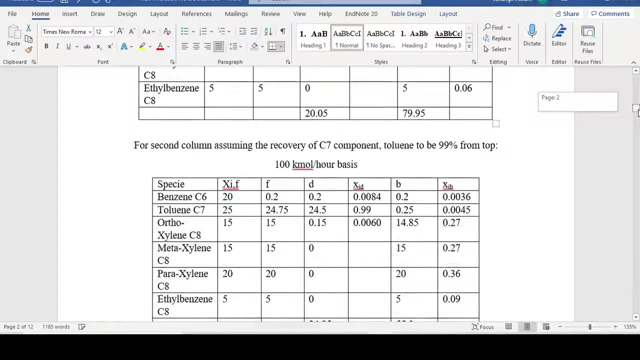 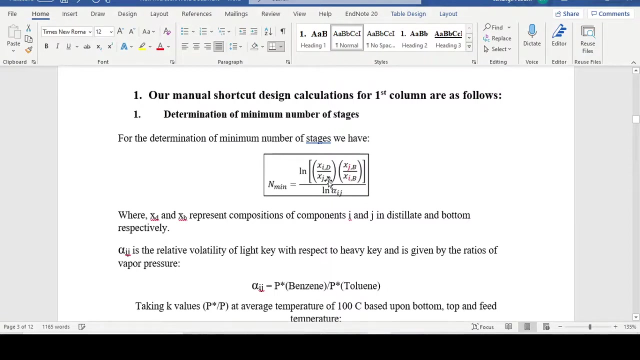 explained later. xid is basically the composition of light key that is desired in the distillate. let's say, we want to get 99 percent separation of benzene in our first column, so xid is basically 0.99. similarly, what will be the composition of heavy key which we desire in the 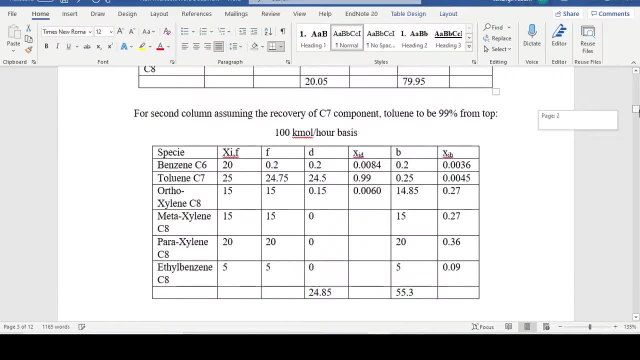 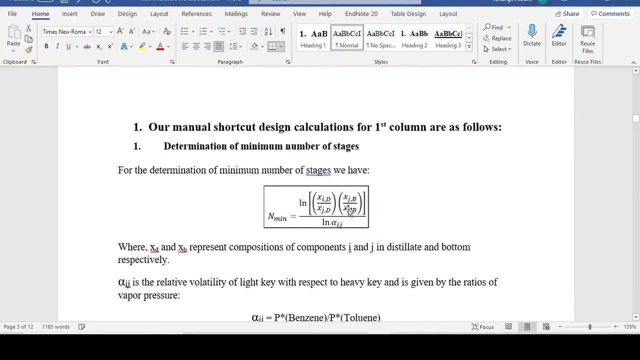 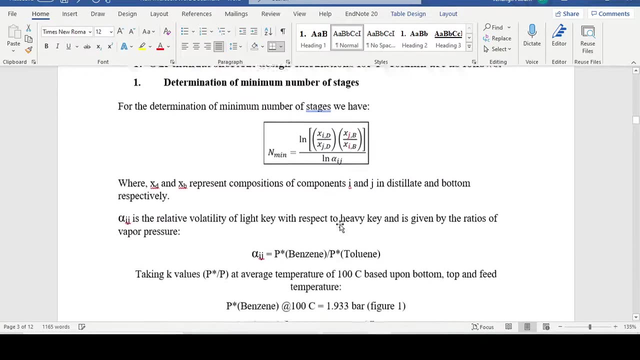 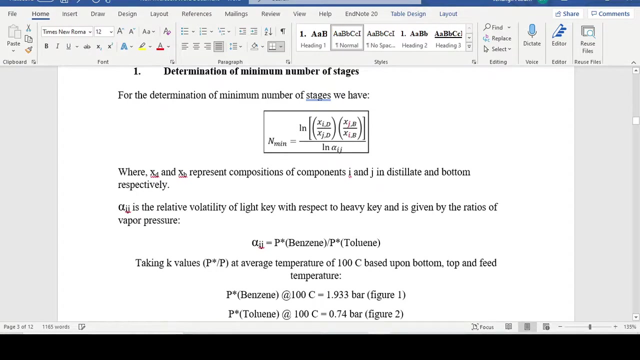 distillate. let's say it is one percent, okay. similarly, we can also mention the values of light in in bottom and heavy key in bottom, and one term is there, which is a relative volatility. so what is relative volatility is relative volatility. ij means relative volatility of i with light key with respect to heavy. 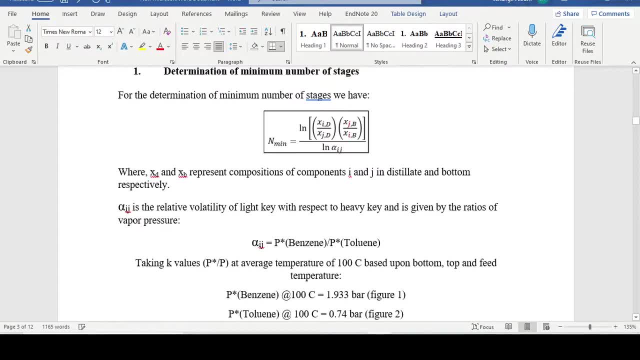 key. what does that mean? relative volatility of benzene over relative volatility of toluene or the heavy key? okay, so it's basically, if we take their ratios, it's basically equal to the ratio of vapor pressure of benzene over ratio vapor pressure of toluene. so basically relative. 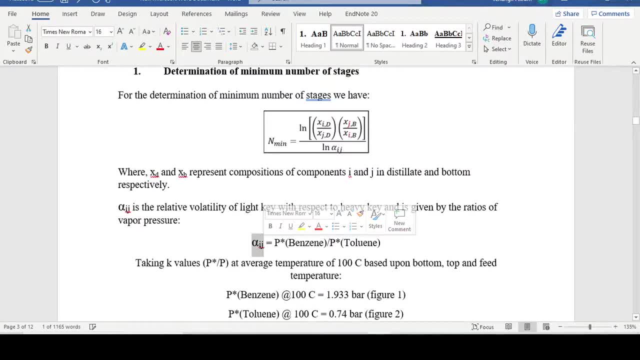 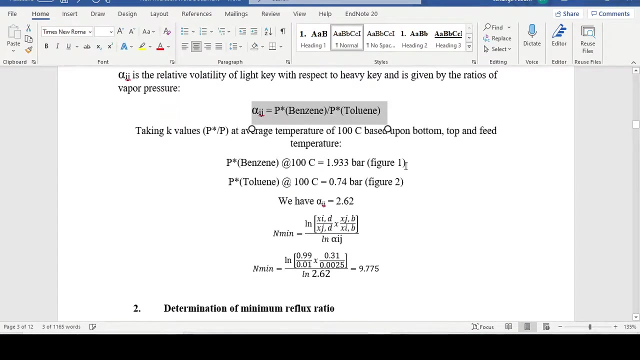 volatility is equal to the ratio of vapor pressure and system pressure and once we have system pressure, overall pressure on both. under both terms, they both cancel out and we can have a correlation which is equal to the ratio of vapor pressures of both keys. okay, so if any one of you have 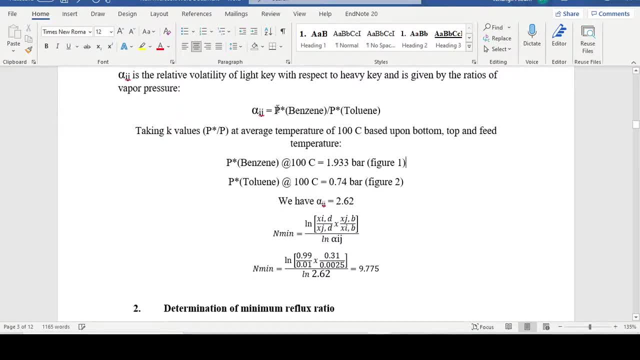 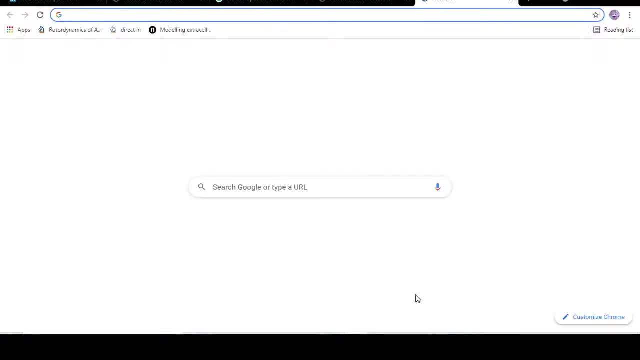 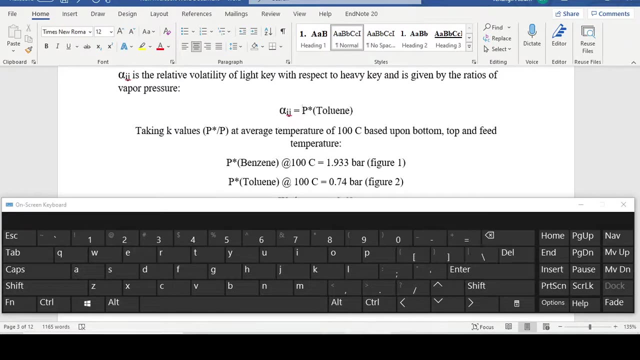 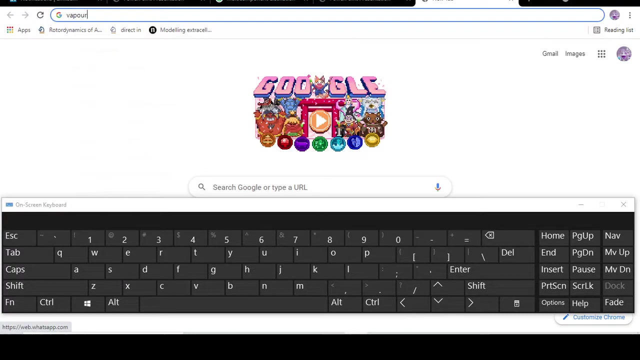 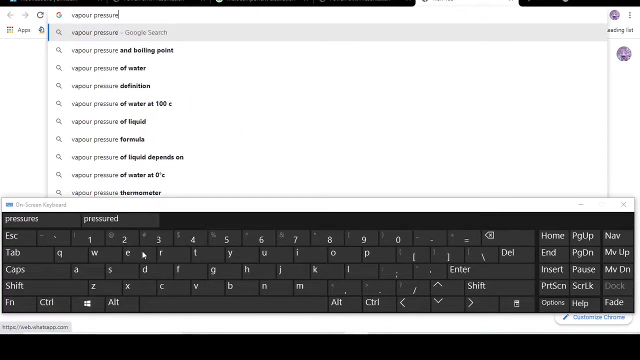 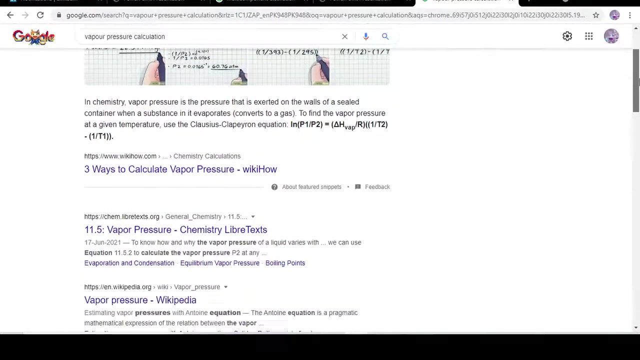 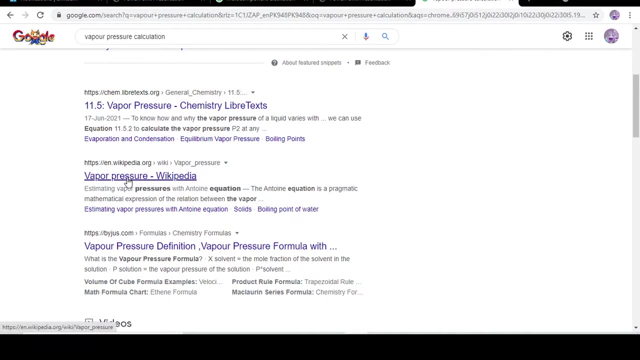 used, uh, has calculated those, these values. i'm- uh, let me recall what was the equation for determination of i i just, it just slipped my mind. what was the name of the equation which is generally used. so you can see here it is determining. okay, let us open wikipedia. 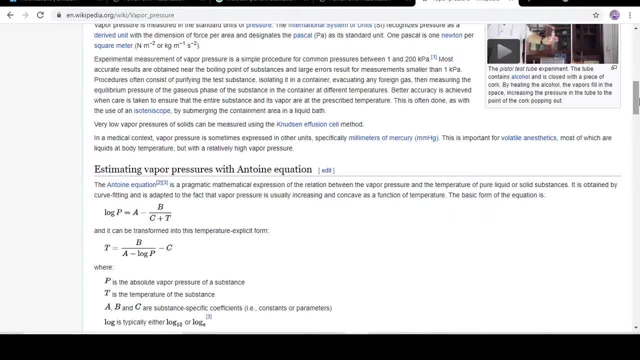 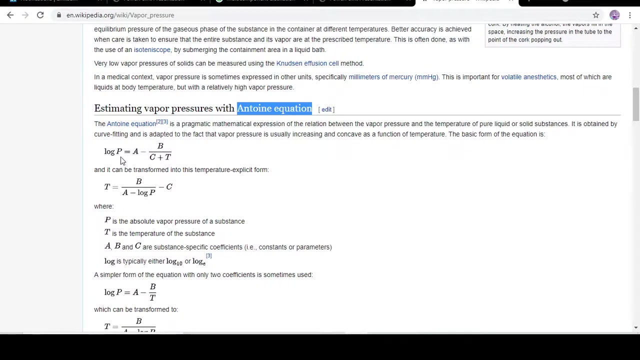 yes, it's basically calculated, uh, through untied equation. so it it has. uh, you can find the parameters of untied equation of any species on google, like you can. uh, there are several thermodynamics website which will help you in getting the value of these parameters, after which you can calculate your vapor pressure. okay, after you have calculated your vapor pressures, 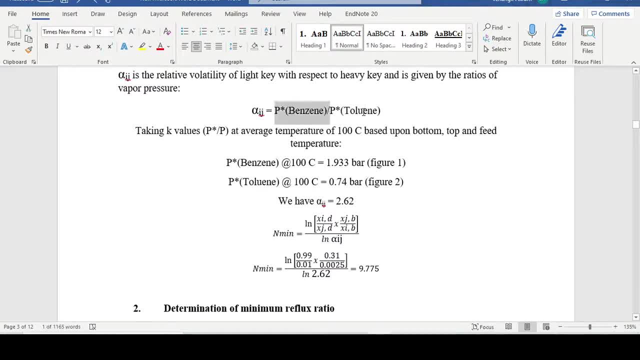 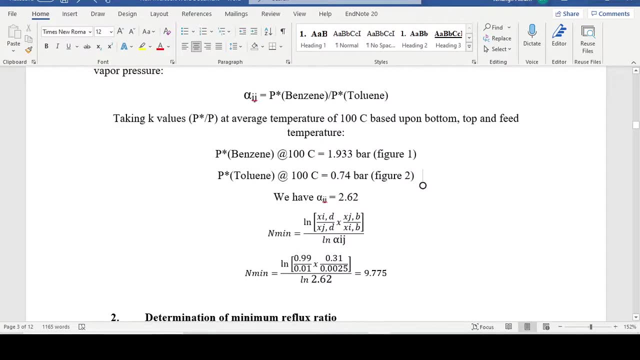 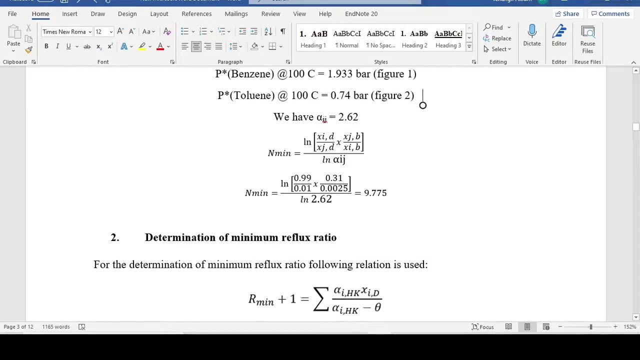 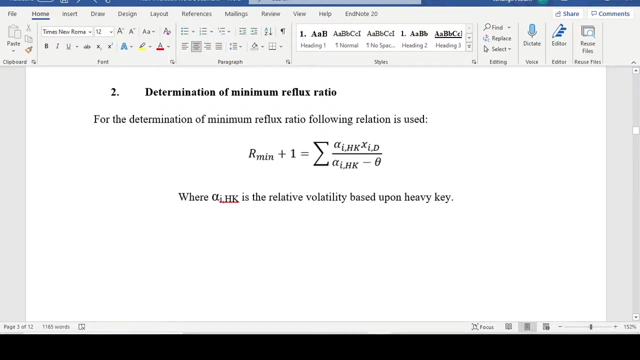 get your, you can get your relative volatility and after you also know that these are based on certain temperature. so you you will have to get the value on system temperature and after using the values in your correlation, you will be able to get your minimum number of stages. similarly, we can, we have as we. 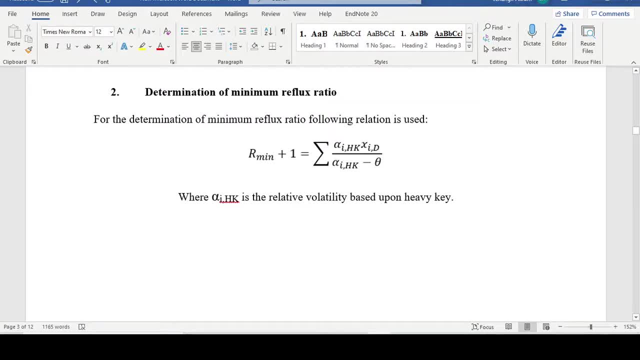 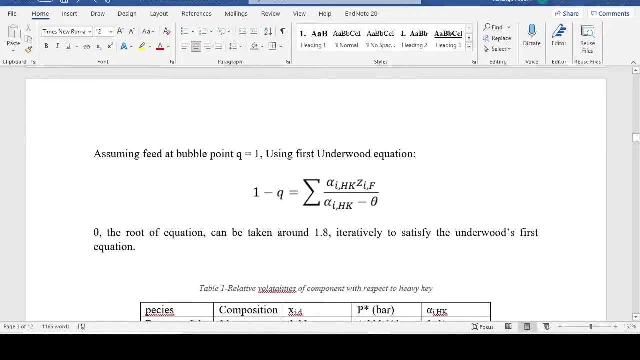 have. we know how to calculate the value of vertical utility. we can tell you the calculation of minimum reflux ratio. so showed you earlier. there are two equations. first, we will solve this equation to get our the value of theta. so what it is doing is that we have. 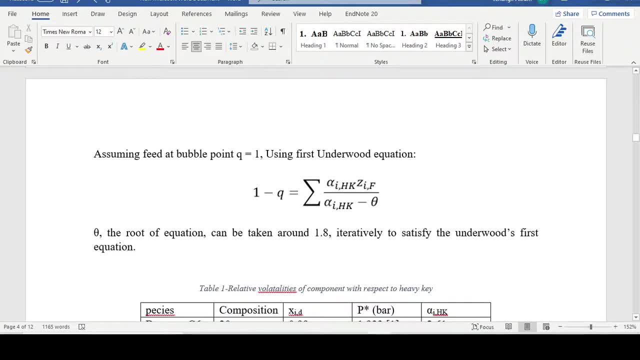 chosen a value, like we. what is the temperature? based upon the temperature of your feed, you can select a feed condition. Q would basically represent the feed condition, same as the Q which is plotted on mole fractions of binary component in k-thela method components. so basically the same Q. you can google how to find the value of feed. 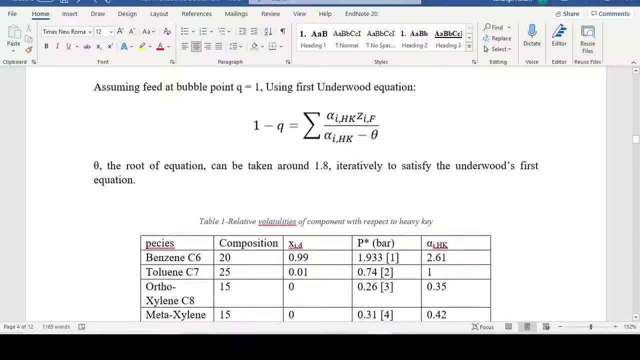 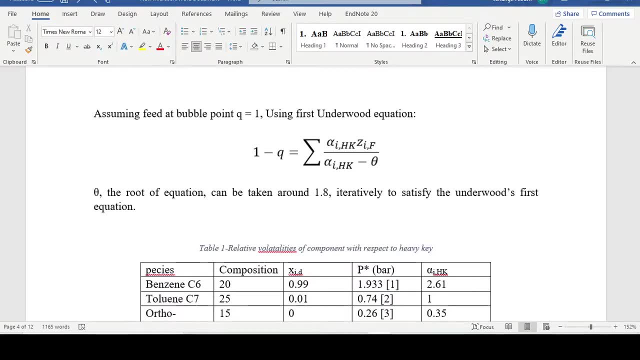 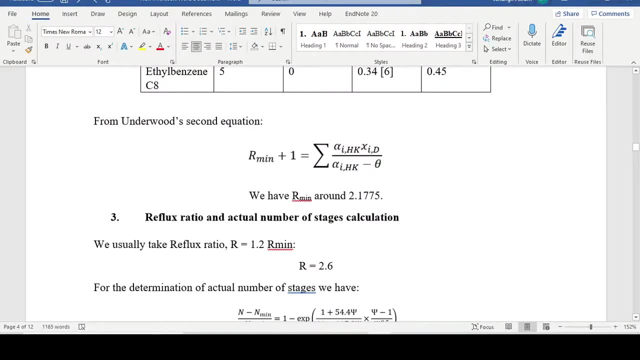 condition. okay, after I can also share the file with you. if anyone will like, I will share the file. and similarly, after inputting the value of Q, you can calculate this theta and after you have got your theta you can put your, put all the values in here and get the minimum reflux ratio. okay, a minimum reflux. 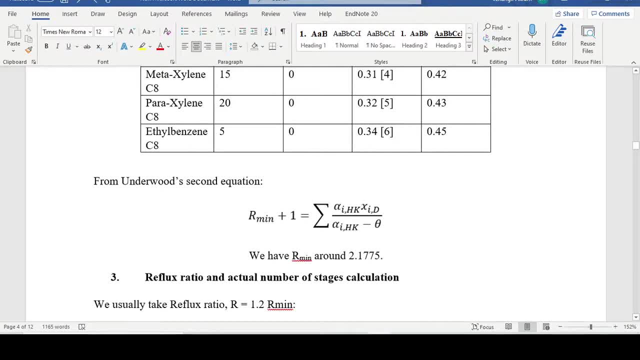 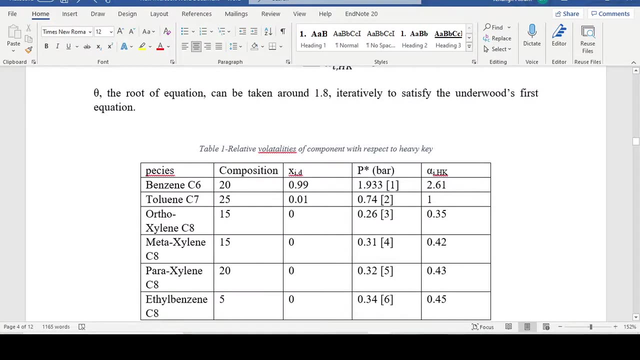 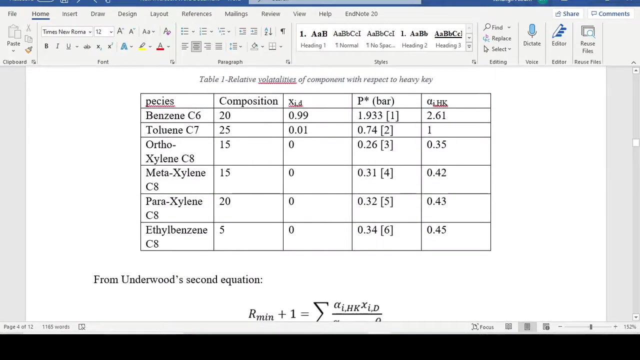 basically this submission terms is term is indicating all is indicating submission, so you don't don't have to worry about anything. you see we have xt composition and, yes, relative volatility of heavy key, basically with respect to heavy keys, are shown in here. okay, as heavy key is tolvain, so relative volatility based upon tolvain for 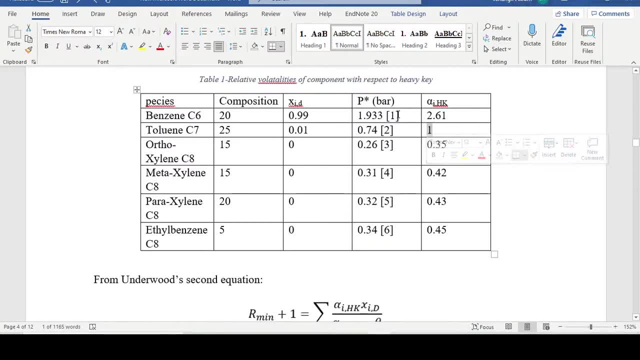 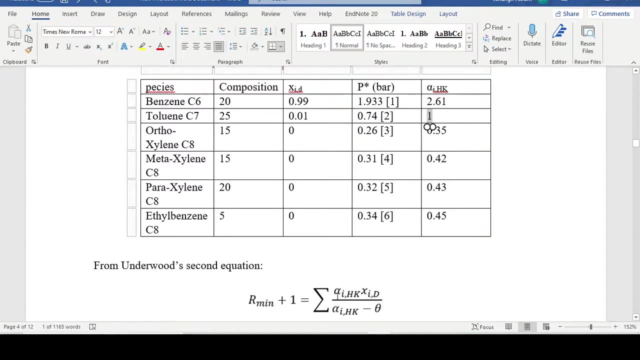 for tolvain will be one for others. like we are dividing all by their partial pressures, uh, vapor pressure- we will get these values and after getting like one, two, three, four, after getting six values, we will add them all. okay, after getting all the seven values, we will. 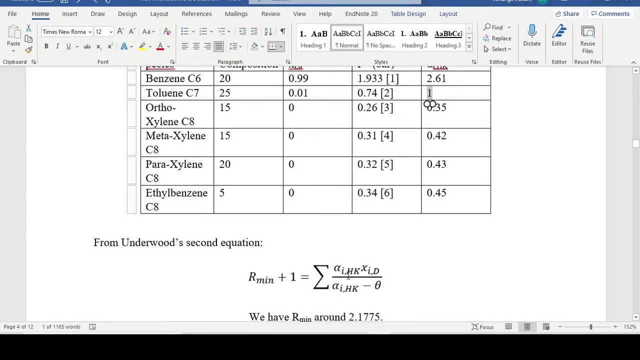 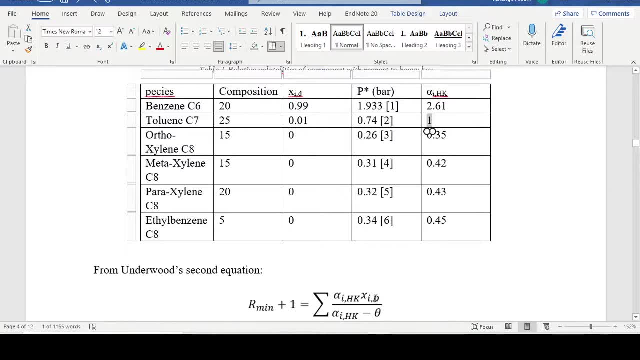 add them all to get this submission term and theta will be same in all the values x, i, d will be, uh, different. basically, it will be zero for these terms and okay. and similarly, after getting these values, we will get our minimum reflux ratio and i, as you know that we convert. 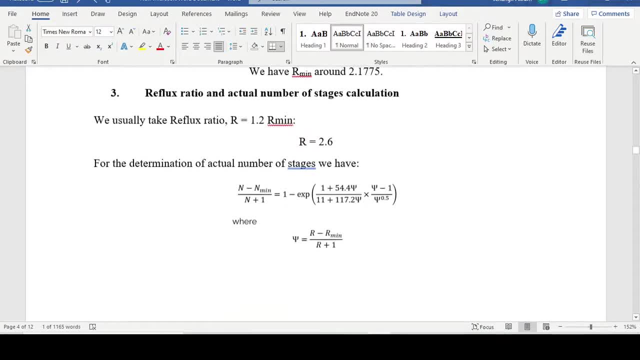 minimum reflux ratio in actual or required reflux ratio, which as a rule of thumb is suggested in stefan hall and other uh guide books to be almost 1.2 times of minimum reflux ratio. like 1.2 is an optimum value for uh adjusting our reflux ratio. so after we multiply we will get our 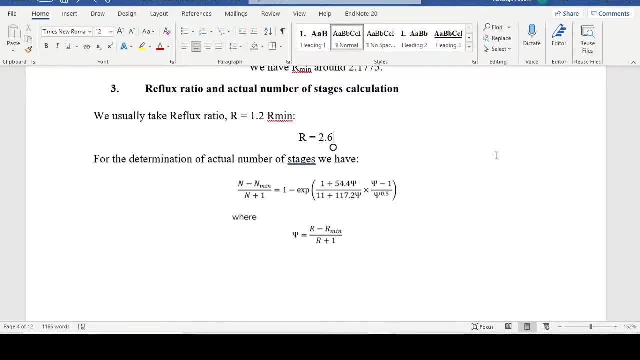 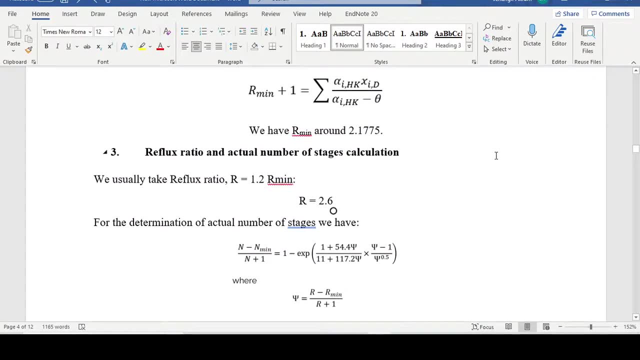 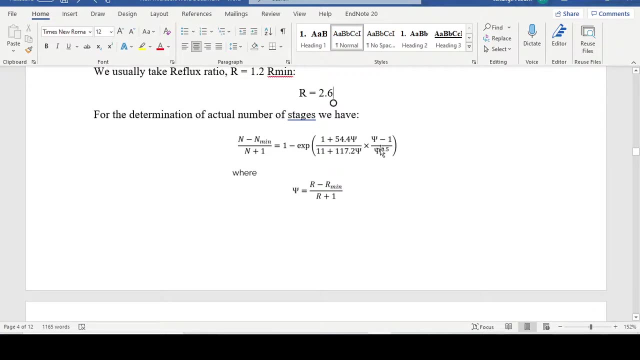 reflux ratios value. okay, and uh, you as you know that we above we calculated minimum number of stages, so we also have to convert that minimum number of stages into actual number of stages. we also have an equation for that. you see, there is nothing new in this equation. we have values of 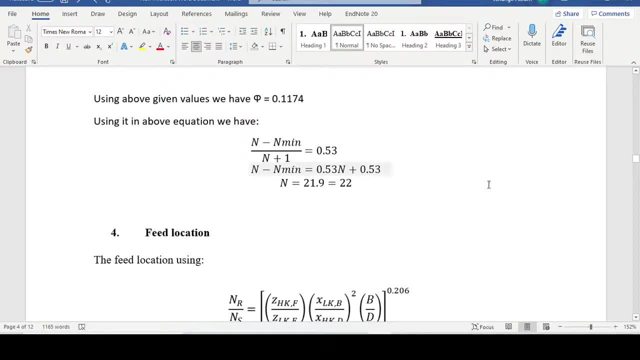 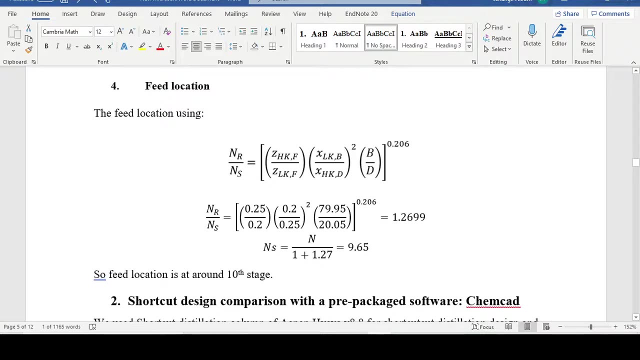 all these parameters. after inputting this value, we will get our minimum number of stages to be- oh, actual number of stages to be almost 22.. similarly, we have another equation. nothing is new in this equation as well: bottom display rate and bottom rate. we have this: 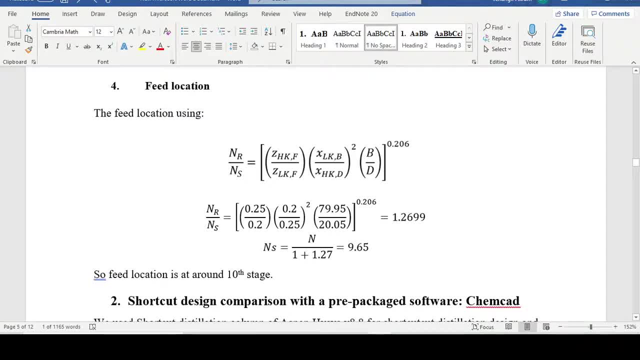 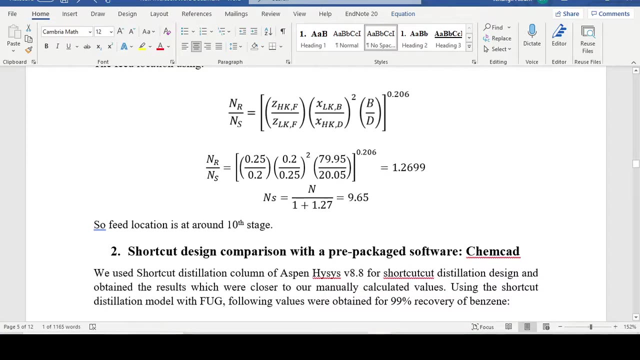 light key in bottom. we have the heavy key in toluene in display and benzene in bottoms and it is basically a toluene in the feed and it is basically a benzene in the field. okay, after inputting value, we will calculate our desired number of oh feed. location of 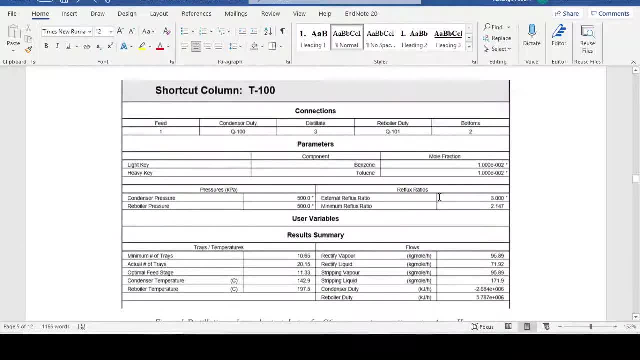 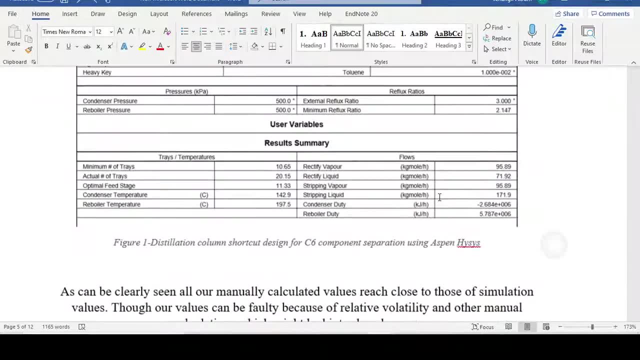 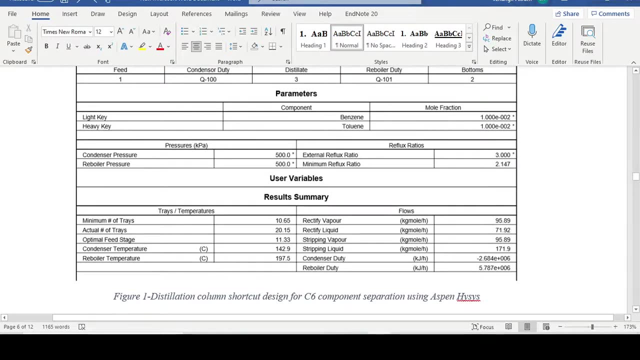 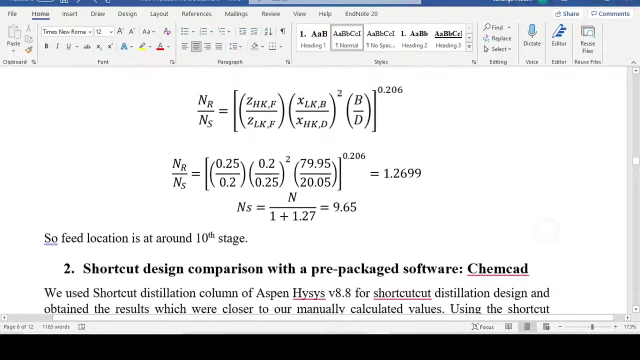 multi-component distillation curve. we also carried out this calculation in aspen, high seas- 8.8, and we got the following values. like you see, minimum number of stages is 10.5, actually is 20.15, in our case it was 22 and feed stage was a 11.33 in their case. 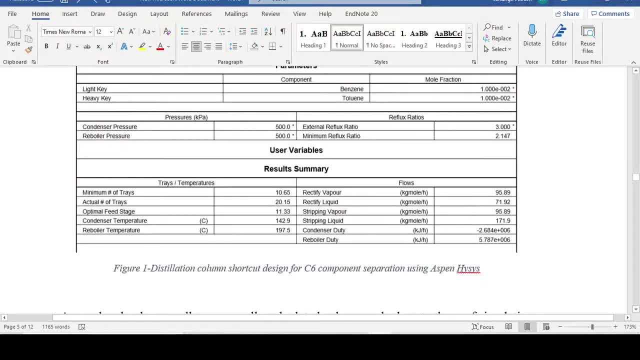 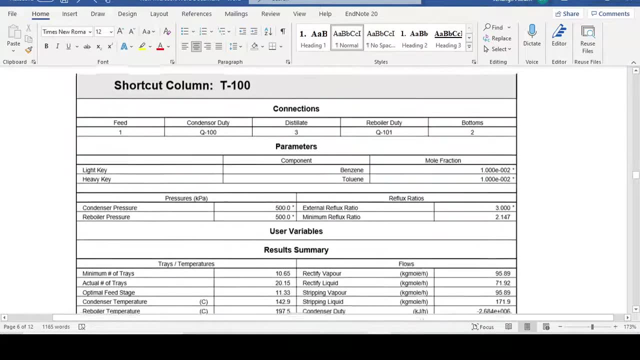 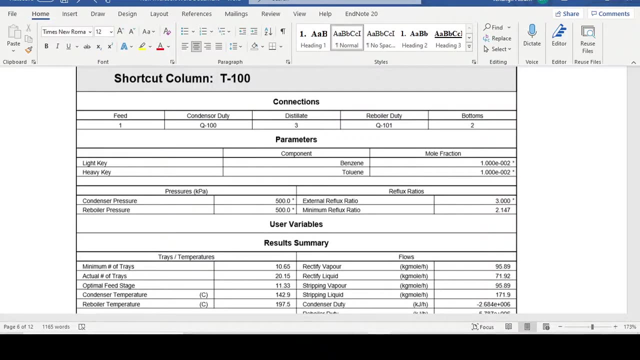 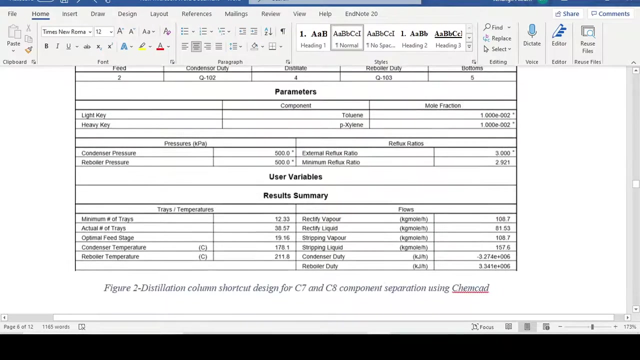 while in our case it was almost 9.65, which is almost 10.. so you can see that aspen is a shortcut palette in, or the shortcut distillation model in aspen, high seas, is based upon these three equations just elaborated. similarly, we can use a second component in which second column you see in this: 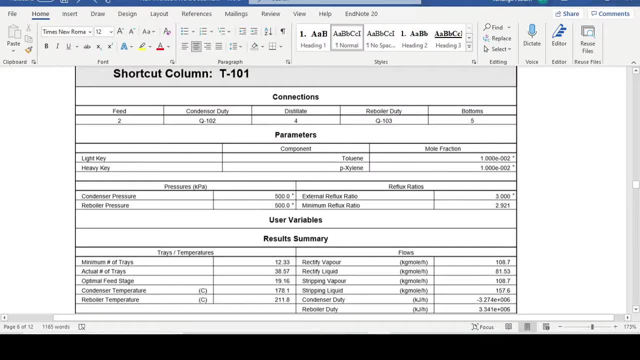 column we have selected, as benzene has already been removed in the second column. so in second column our light key will be the toluene and heavy key will be the xylene, and so we can carry out further a separation in our third column, where toluene will be the most concentrated. 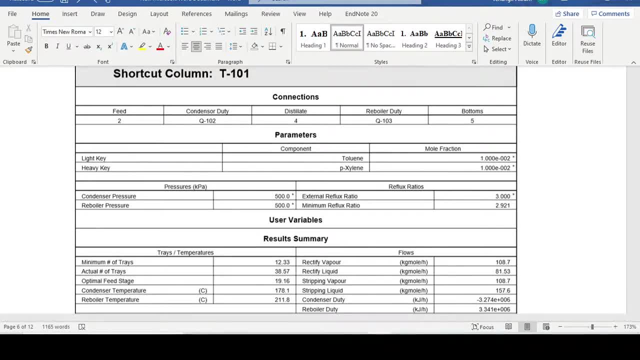 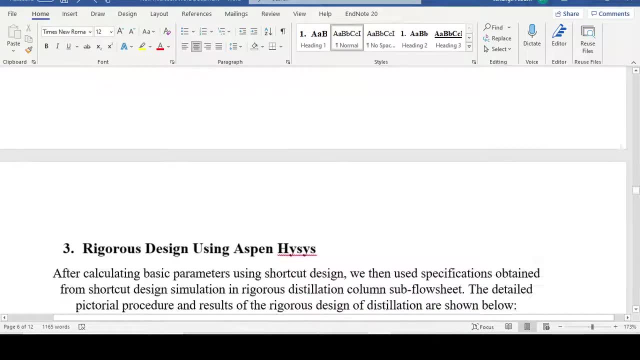 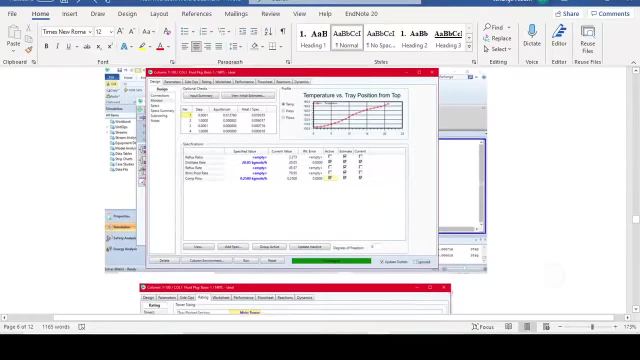 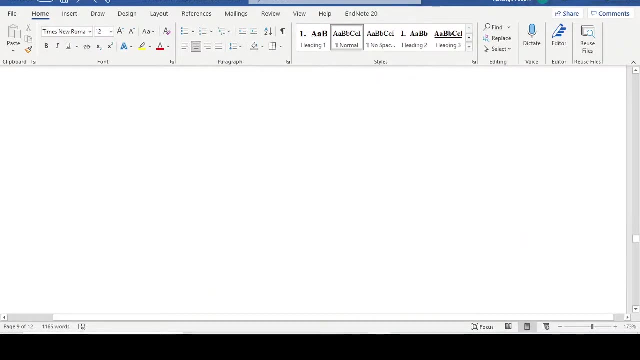 product of our distillate, while all those heavy keys containing carbon eight atoms will be living through the bottom. similarly, we can also carry out a rigorous design in aspen high seas, which you can try yourself, because all the major values which are needed are already given by the shortcut method. so what we do is that, first of all, we design. 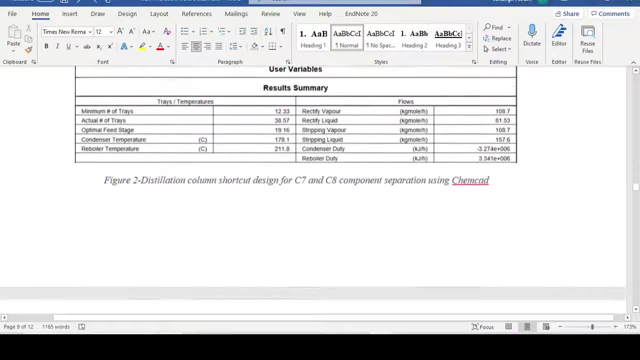 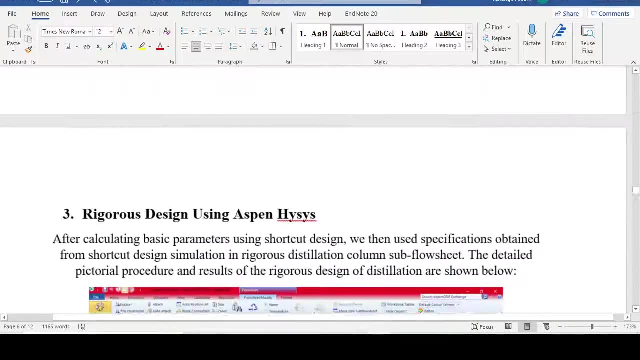 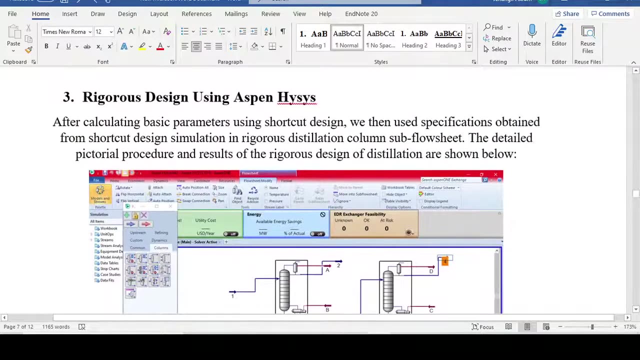 a shortcut distillation column using fug method. okay, after we have carried out the calculations, such as minimum number of trays, actual number of trays, minimum number of stages, pressure conditions and all those conditions, we will be using a rigorous model. so for the calculation of rigorous model, you see, 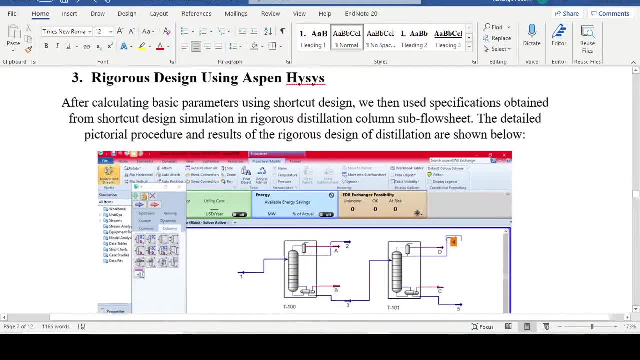 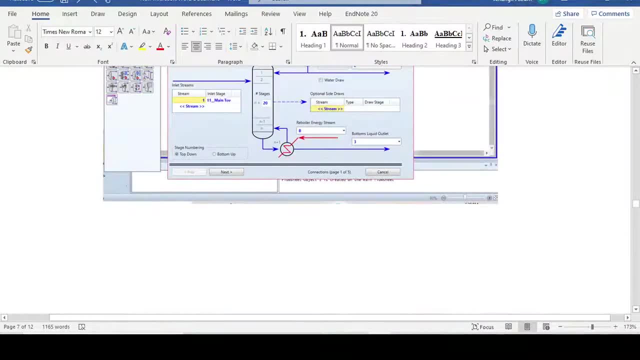 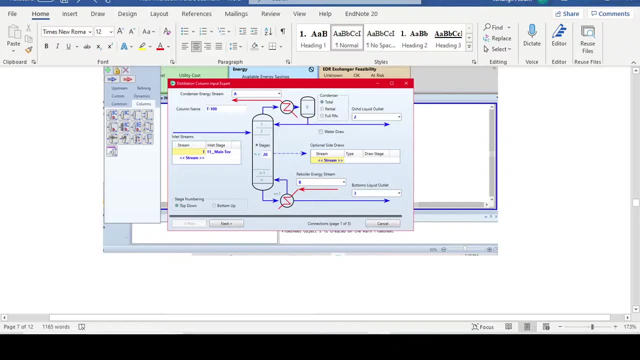 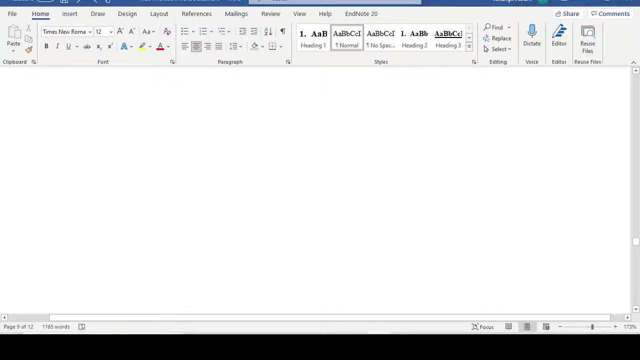 there is nothing, i think there is nothing obtained. for, you see, we will input all the values which we got from there, like we found that minimum number of stages was almost 20- let's say our feed feed stage was 10- and after inputting all the values and we will be able to design a rigorous model in our aspen high seas, 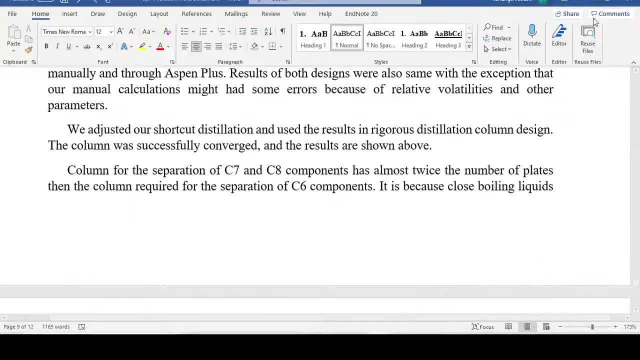 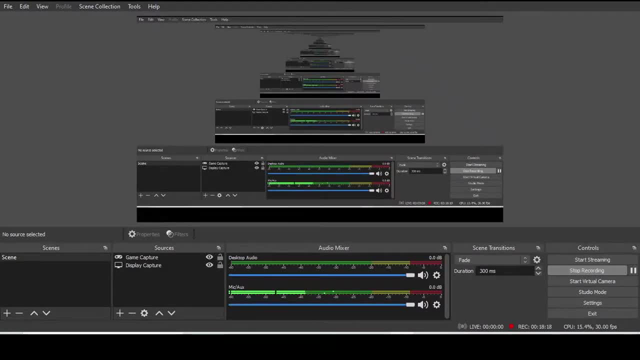 okay, you see hope. so you enjoyed the video and actually, and please try the aspen high seas part yourself, if you remain enabled, uh, to use aspen hyacinth, let me know. i will create a separate video using aston hysナis for the design of regress distillation. 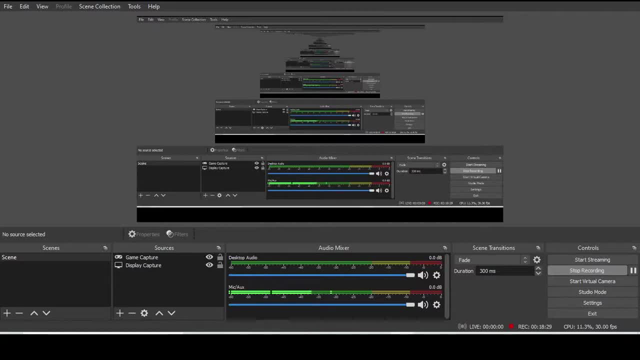 column. but i will suggest you first of all carry out the calculation manually, like as i explained how to use the stimulation, learn how to use those equations. after you have a learned, then move on to the s1 hisis part and try the rigorous model later. hope you enjoyed the video. 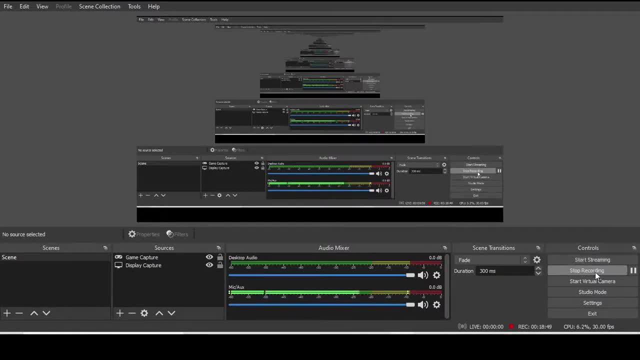 and learned a lot from this short video session and please don't don't forget to subscribe my channel. thank you.